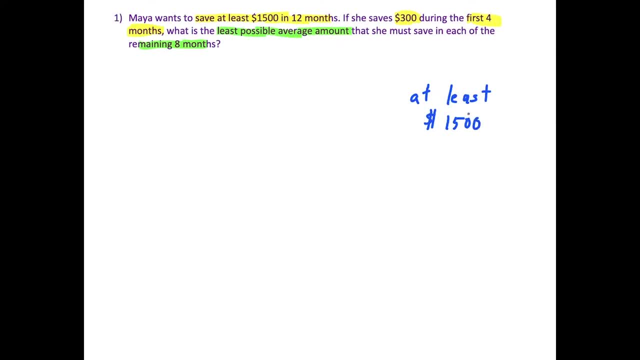 phrase at least: if Maya wants to save at least $1,500,, at least $1,500,, at least $1,500, then she either wants to save exactly $1,500 or more than that. So the amount that she has to. 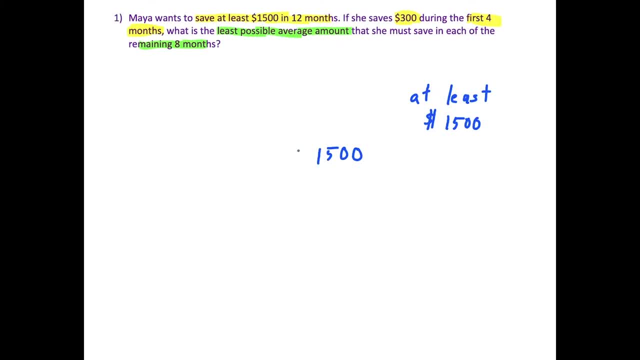 save. we're going to write an expression over here on the left, but that amount has to be greater than or equal to $1,500. Because, remember, at least means $1,500 or more. So the left side is greater than or equal to $1,500. And we're told here that she already saved $300.. So that 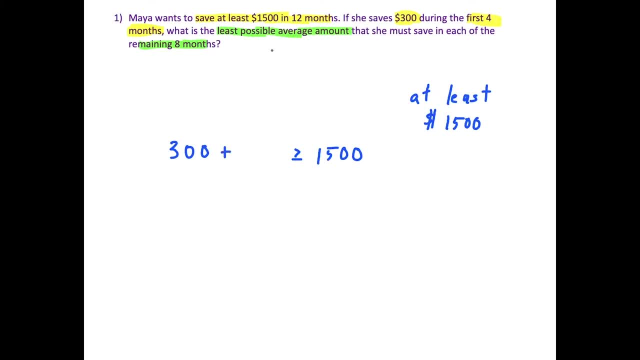 amount is fixed Plus, and the question here is: is Maya going to save at least $1,500? And the question is: what is the least possible average amount that she must save in each of the remaining eight months? So if we define the variable x here, 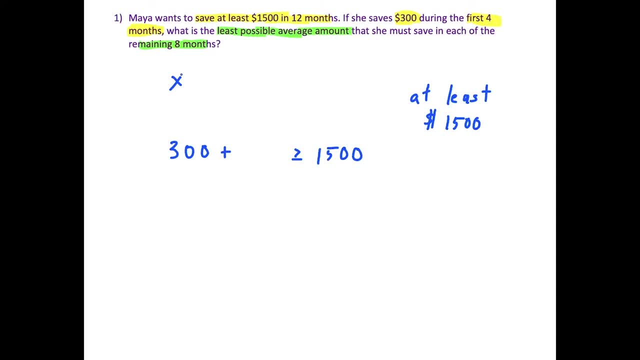 x is going to represent the average amount of money Maya saves in the remaining eight months. So if we think carefully here about how we defined x, well, if there are eight months remaining, then to find out how much Maya saves in the remaining eight months, we're going to multiply. 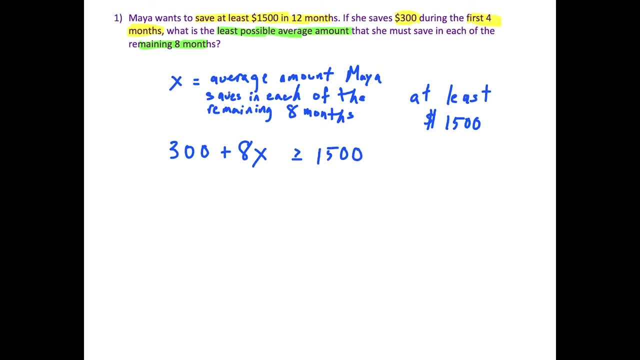 eight times x, Because if she saves x dollars on average each of the remaining eight months, then if we multiply x by eight, that tells us how much she saves in the eight months in total. So then, to solve this question here, all we have to do is just 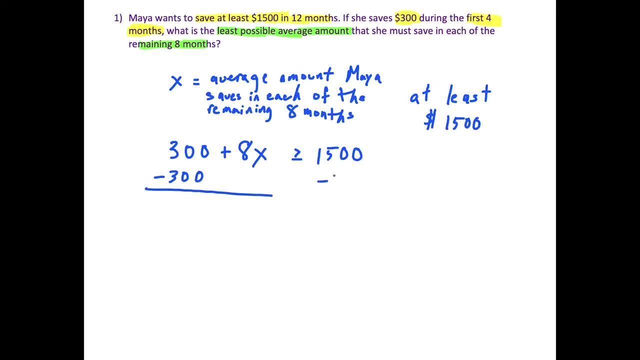 we'll solve the inequality. we're going to subtract 300 on both sides And now we've got 8x. x is greater than or equal to 1,200.. And then to solve for x, we're just going to divide both. 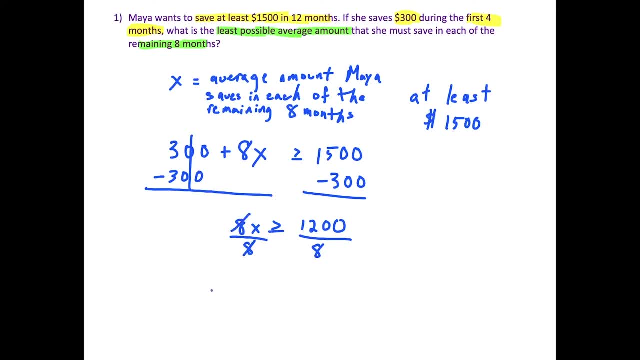 sides by 8.. And now, when this simplifies, here we have: x is greater than or equal to, 8, goes into 12 once with a remainder of 4, and 8 goes into 40 five times, and then 8 goes into 0,, 0 times. 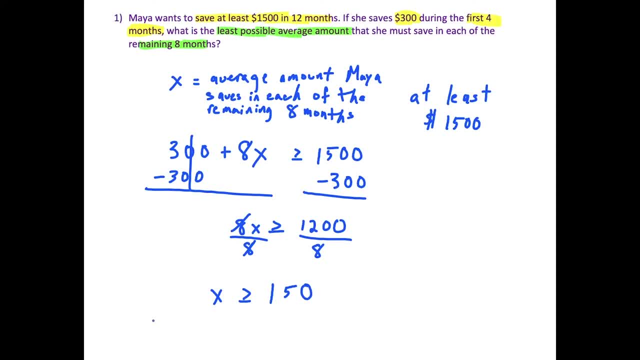 So now we just have to interpret this answer. If x is greater than or equal to 150, in the context of the question, Maya has to save an average amount of at least $150 a month for the remaining eight months in order to reach her goal. Okay, so take a moment to read through the second question. 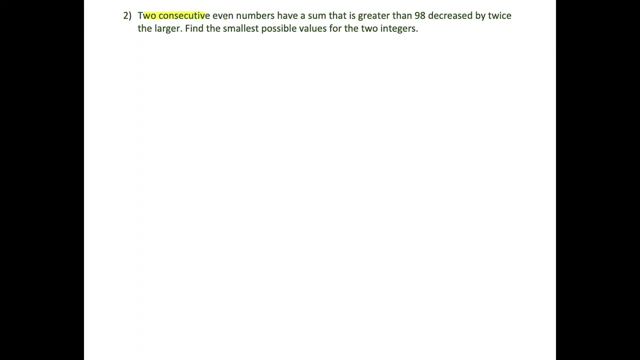 And what we're looking for here is we want to find two consecutive even numbers that have a sum that is greater than or equal to 150. And so we're going to take a moment to read through this second question, And now this part's a little wacky. The sum has to be greater than 98, decreased by twice the larger and the larger. 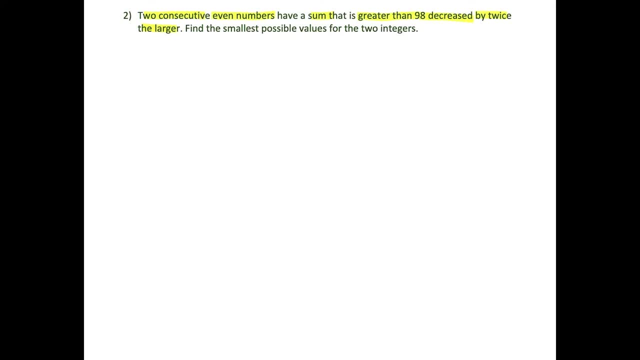 what we're talking about here is the larger even number, And the task here is to find the smallest possible values for these two integers. So I mean we essentially highlighted the whole question, but I guess it is all important here. So we need to define some variables. we're going to say: let x equal our. 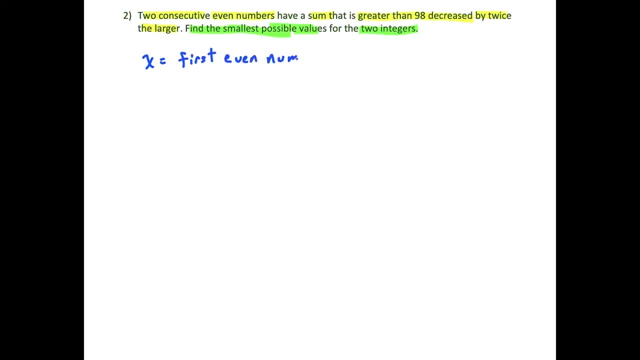 first even number And then for the next part here if they are consecutive even numbers. so this is what we have to think about. If I list a bunch of even numbers here and I could start at zero, but I'll start at two. The pattern to go from one even number to the next one consecutive. 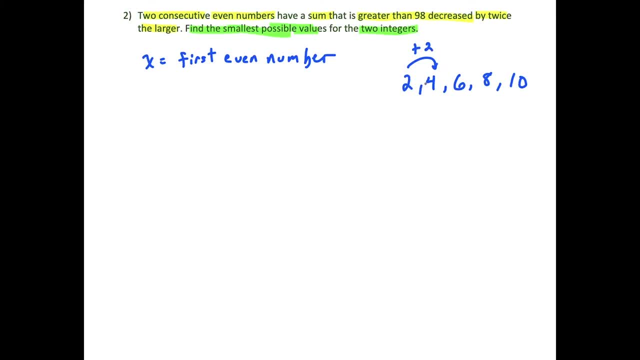 means the one right after So, one right after another. we're not skipping four or skipping six, But to go from one even number to the next, we are adding two. So that means, if x equals our first even number, then x plus two is going to be our second even number. 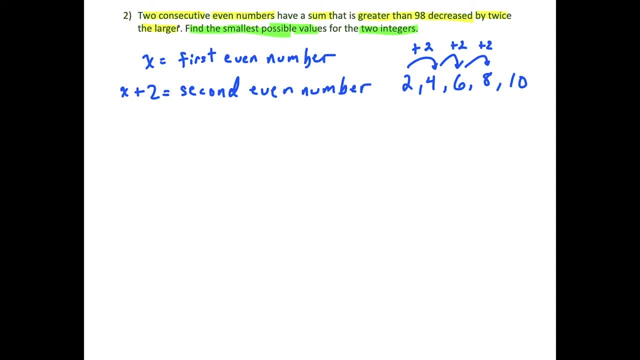 So now let's apply this to the details in the question. They're telling us that the sum of these two consecutive even numbers, So what we're going to do here is add them together, We're going to have x plus. the second number is x plus two. 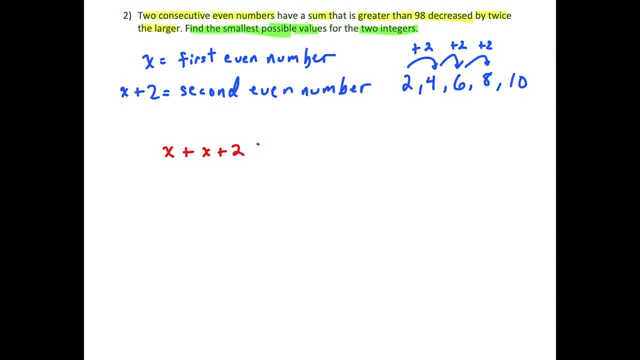 And we're saying here that it is greater than. So we're going to throw in our greater than symbol. And now we have next 98 decreased by. This phrase here tells us to subtract. Okay, so this is just a different way of saying subtract. So we're going to have 98 decreased by twice. Twice means. 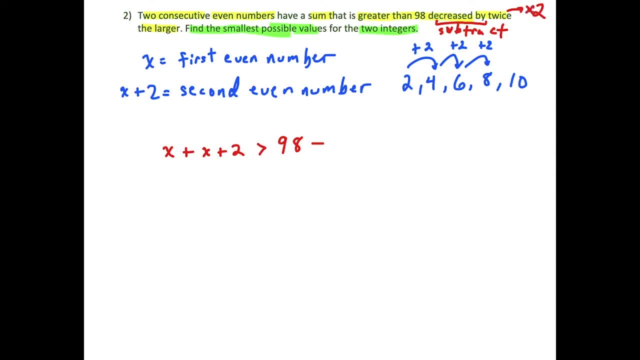 times two. So we're multiplying by two. We could put a multiplication sign here. So minus two times the larger. And if x is our first even number, the second even number, this is the larger of the two because it has it's plus two, right. 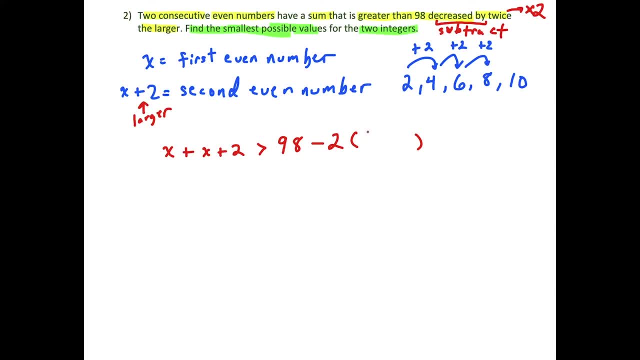 It's a greater number because two is added to it. So that's what's going in parentheses. here is the x plus two. So just so we're clear on all this: 98 decreased means subtract, And then twice means multiply by two. 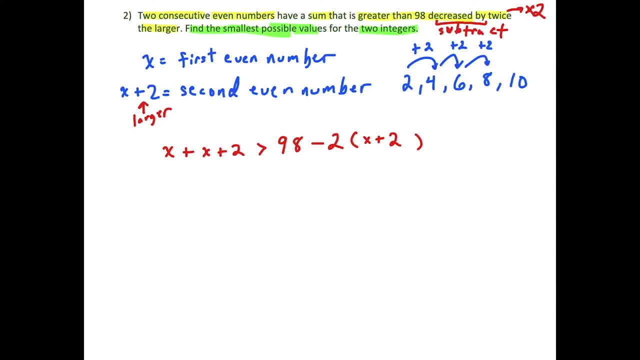 The larger even number is x plus two. So then all we have to do here is solve this inequality. So x plus x simplifies to two x. we have two. x plus two is greater than 98.. And I'll be careful here. 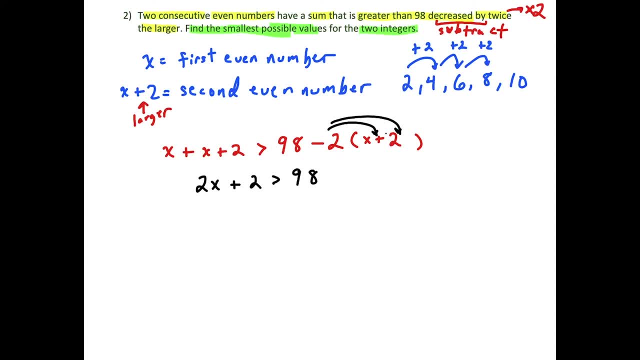 we're distributing a negative, So we have to make sure we change the sign both times. So we have minus two x and then negative two times. positive two is negative four. Then from here we're going to get the x's on one side. 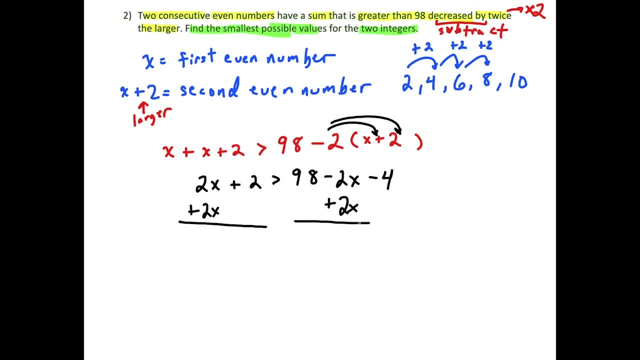 So we could go ahead and add two x to both sides. Now we've got four. x plus two is greater than, and we can combine like terms: 98 minus four is 94. So then the next thing we want to do is subtract two on both sides And we've 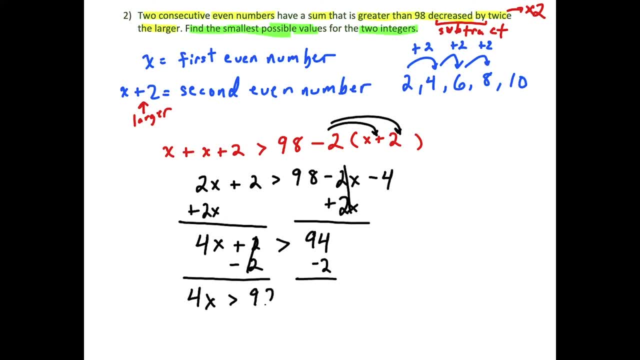 got four. x is greater than 92. So then, once we solve for x here, we'll see how this works out, And we're going to let this getatempent around two times And we're going to write the result over here. 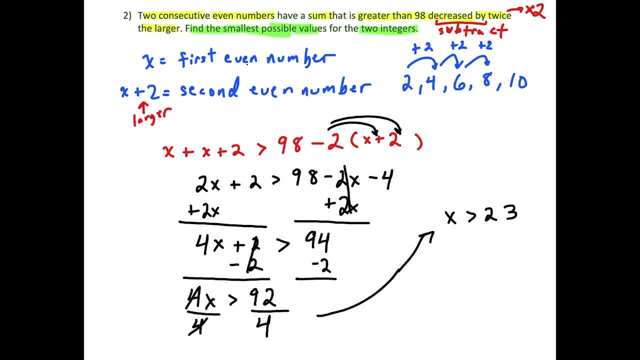 that x is, And those two x's that are not equal to x aren't equal to twelve or more to twelve. so that'll be the result And we'll write the result over here. that x is 92 divided by four is twenty-three. Now you might be looking at and saying, oh, wait a minute. and saying, oh, wait a minute. x is supposed to be even. But let's think very, very carefully about this. Now we have to interpret our answer. You should be asking yourself what is. greater than twenty-three. Now to look at this, you want to know that what is the next integer? twenty-four is same. Well, the next integer twenty-four is same, greater than twenty-three, So x. in this case, we want to find the two two times. 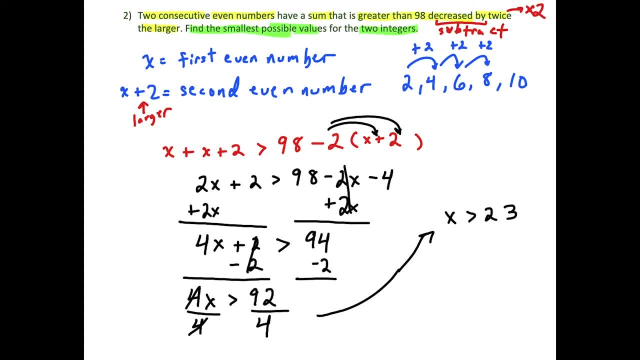 the two smallest possible values, or the smallest possible values for the two integers. So we're going to say here that the first number, x, is equal to 24.. And then, if x equals 24, then x plus 2 is going to be 26.. So these are in fact our two solutions. But now let's go ahead and check. 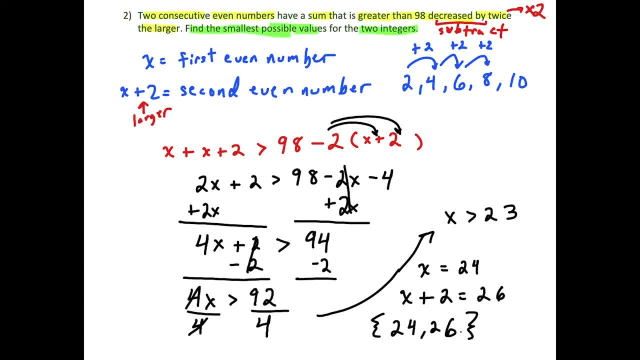 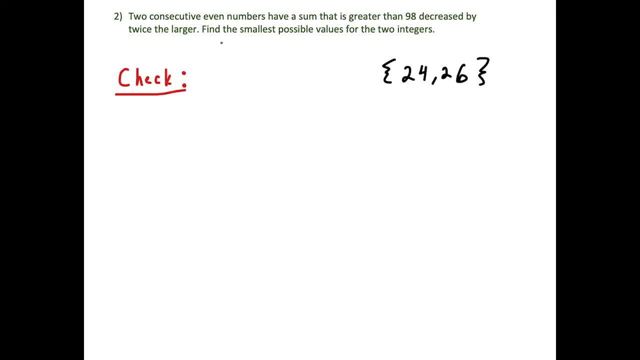 We're going to verify here that these two do in fact check out. Okay, so now let's check our answer And let's throw our solution set back into the word problem. So we have the sum of these two consecutive even numbers. So we're going to add our consecutive even numbers 24 and 26.. 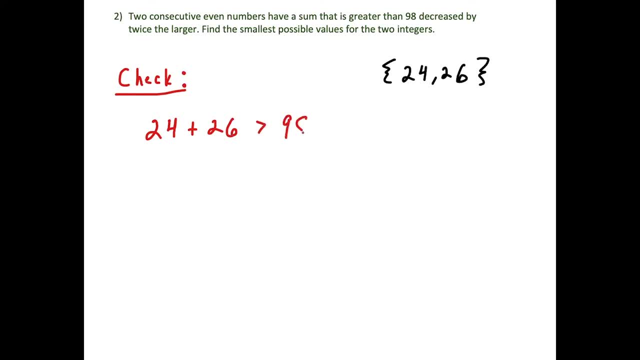 And it's going to be greater than 98, decreased by twice the larger And the larger of the two numbers is 26.. So now, when we simplify this here, 24 plus 26 is 50. And the question is: is 50 greater than 98? minus 2 times 26 is 52. So when we simplify the right, 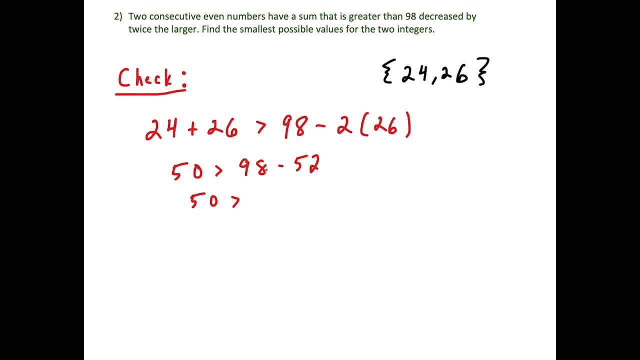 side we have 98 minus 52. And we'll subtract the ones, 8 minus 2 is 6.. 9 minus 5 is 4. And this is in fact true. 50 is greater than 46. So these numbers do check out, But what we have to also. 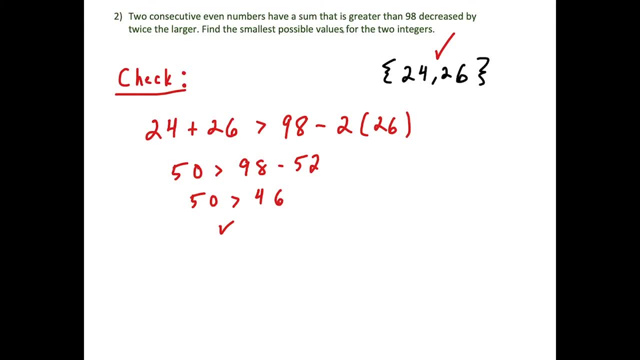 verify here is that these are the smallest possible values for the two integers. So the next thing we should check here is: well, what about the next two numbers down the list? If we were to go with 22 and 24, these two consecutive even numbers are smaller than. 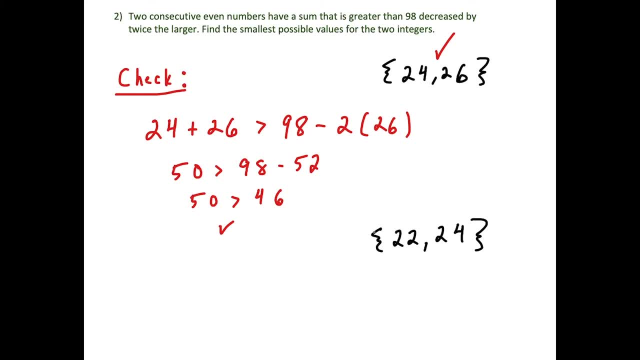 this pair, This is the next pair down the list, And then it would be 20 and 22.. But let's see what happens when we plug these particular values into the question. Well, we have: the sum of these two numbers is 22 plus 24.. And we want to know: is this greater than? 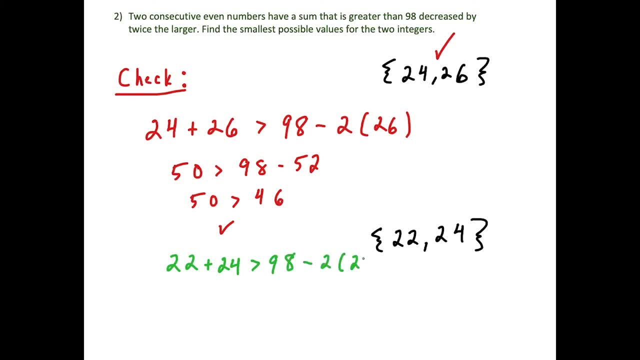 48 decreased by twice the larger, And the larger of these two is 24.. So if we work this out, 22 plus 24 is 46. And we have 98 minus 2 times 24 is 48. But when we simplify this, you see how we get 46.